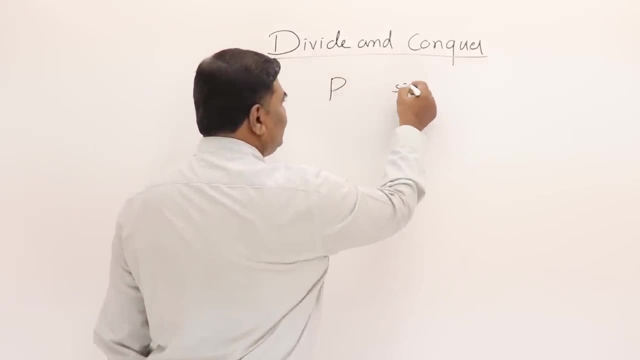 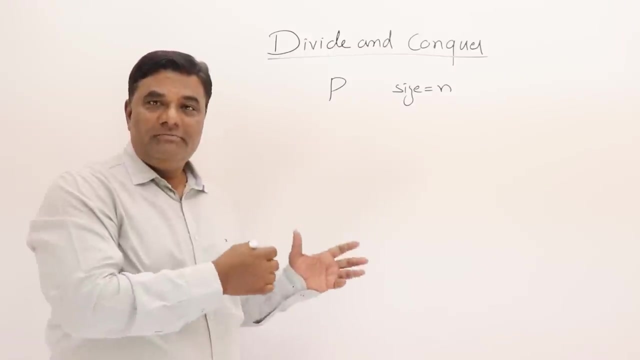 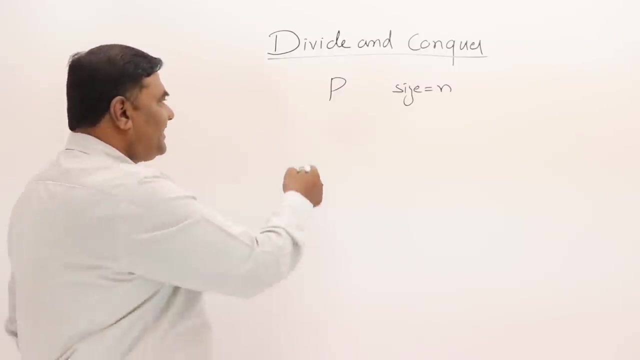 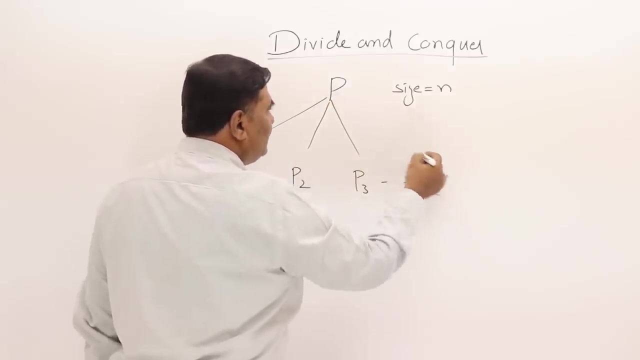 If a problem of some size is given, let us say size is n, This size is n. This is the size of the input for a problem. So if a problem p is there of some size, and if we say that this problem is large, then you can break this problem into smaller sub-problems- p1,, p2, p3, goes on. as many problems as possible. that depends on you. 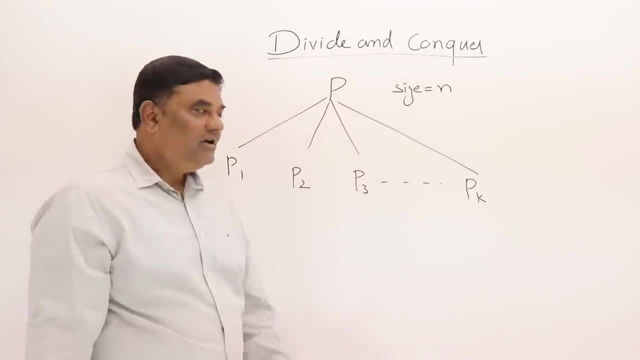 So let us say k sub-problems. Now the large problem is broken down into smaller sub-problems. So the size was larger, so we have broken into smaller size problems. Now these problems, sub-problems, can be solved to obtain their solutions. 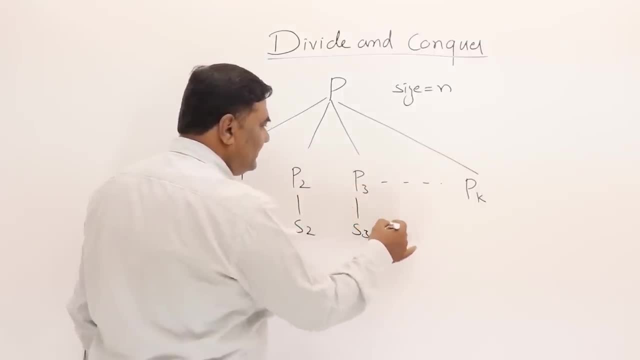 So for this solution 1,, solution 2, and solution 3, and so on, for this solution k, All these are individually solved. Now, once you have the solutions for these, you can combine these solutions to get a solution. 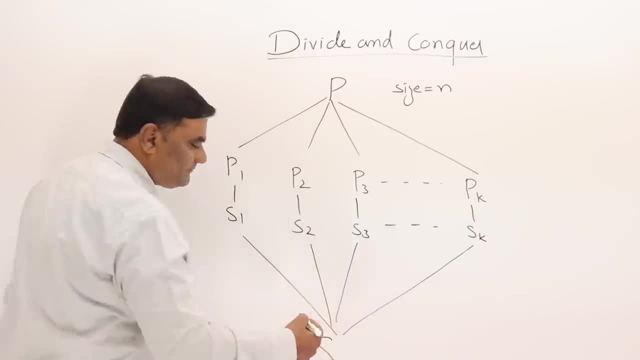 solution for main problem. So if a problem is large, divide the problem into subproblems and solve those subproblems and combine the solutions of subproblems to get the solution for main problem. So it means if a problem cannot be solved, if it is too big, break it into subproblems and solve it. If a 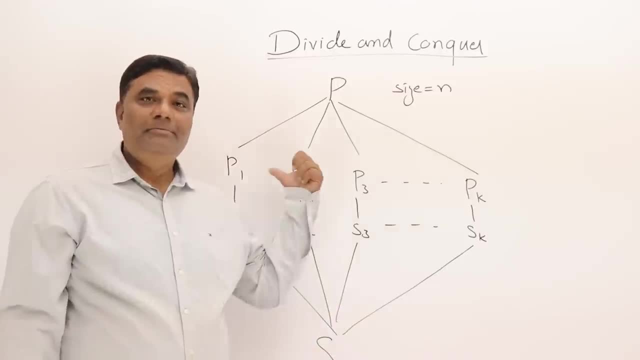 subproblem is also large, then do the same thing. apply divide and conquer strategy on subproblems also. If it is large, again do the same thing: break it into sub subproblems and find the solutions, combine the solution. Now one important thing about divide and conquer: Whatever the problem is the subproblems. 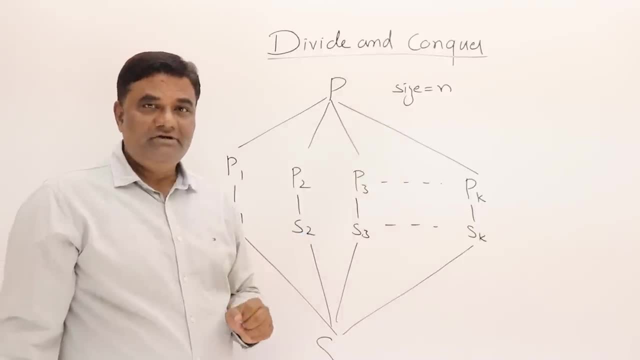 will be same as that problem. For example, if problem is to sort, then the subproblems should also be sort. Or each and every subproblem should be sort, only It cannot convert into some other problem. Like example if problem is. I'll take some real example. if a problem 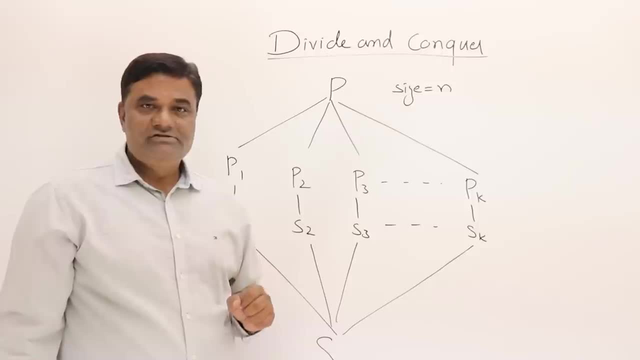 is to conduct a workshop at a college, then it's a big work, so you can divide the work: Preparing invitations, preparing posters, inviting guests and inviting resource persons, arranging resource person: it's a different task. Each is a different task. No, this is not. 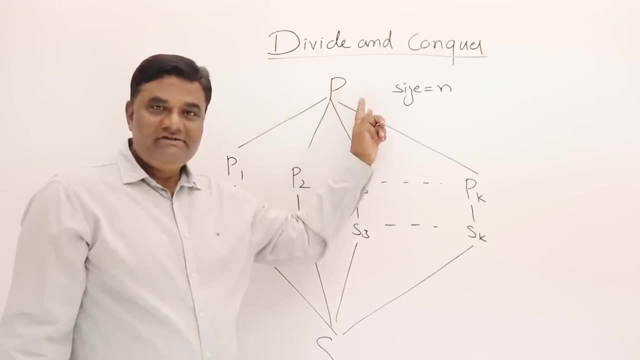 divide and conquer. If, example, this is sort, then the subproblem should also be sort. only Then we call it as divide and conquer strategy. So if a major problem cannot be solved, divide it, and those problems should also be same. So this how? 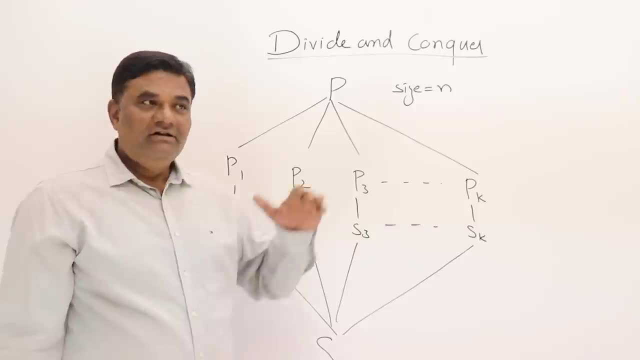 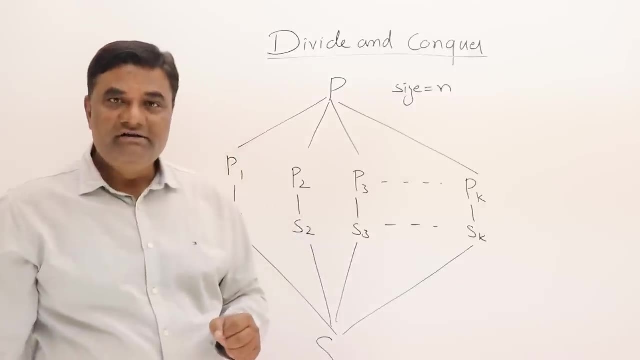 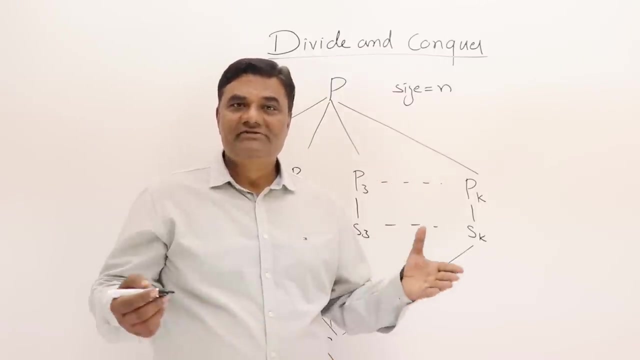 it is recursive in nature. Like this problem is sorting, then these problems are also sorting. So divide and conquer algorithms when you write, or strategy when you take, it will be a recursive. So it says that you recursively solve the problem. If it is too big, recursively solve it. And one important thing is: when you have 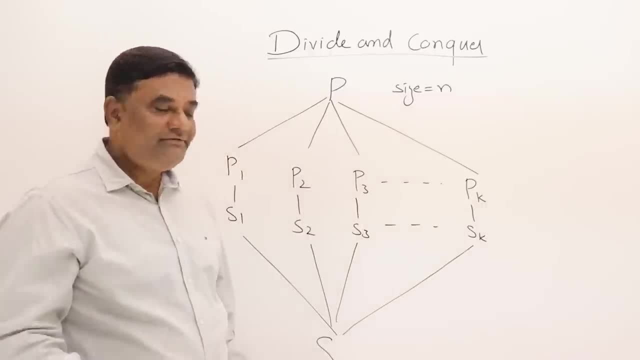 broken the problem into subproblem. you should have some method for combining their solutions to get a main solution. If you are unable to combine, then you cannot adopt this strategy. So this is a guideline. you can see, If you have a problem, how you can understand. can I apply divide and conquer on this one? 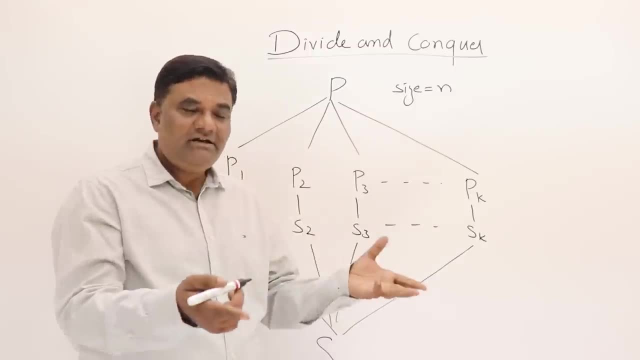 or not. So if you break it, the problem should remain same. Then you can apply divide and conquer, Or you should keep it same. Then divide and conquer strategy is applicable And you should have a method for combining them. So this is the approach of a divide. 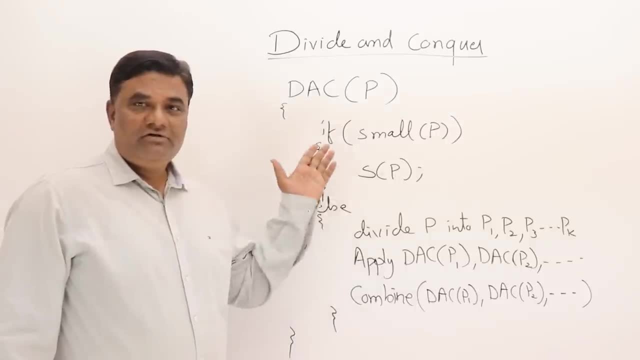 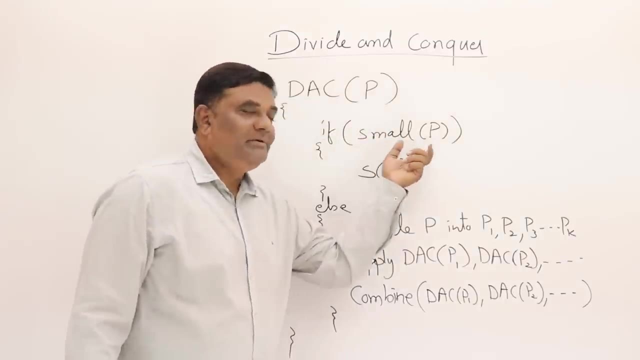 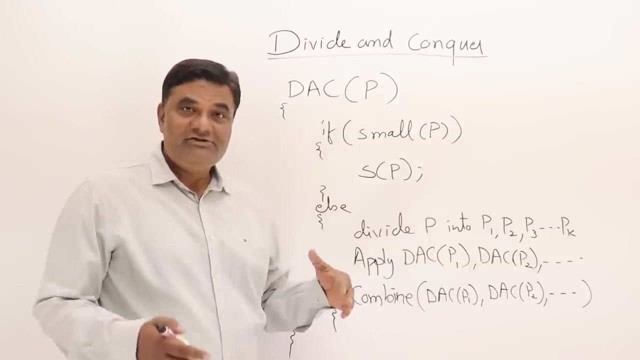 and conquer strategy. Here is a general method for divide and conquer strategy. Divide and conquer upon a problem. P. If the problem is small, then directly solve it. Yes, definitely there must be a solution for small problem. If it is large, you are breaking it. If it is small, then what Solve? 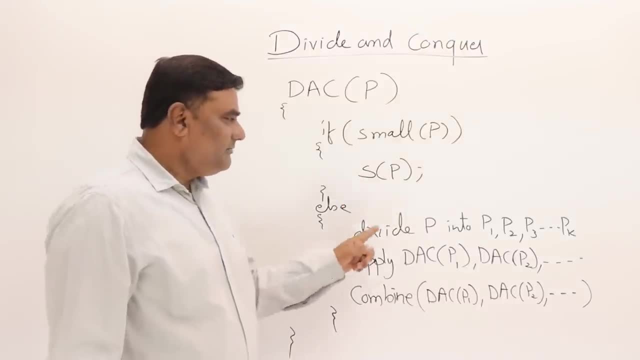 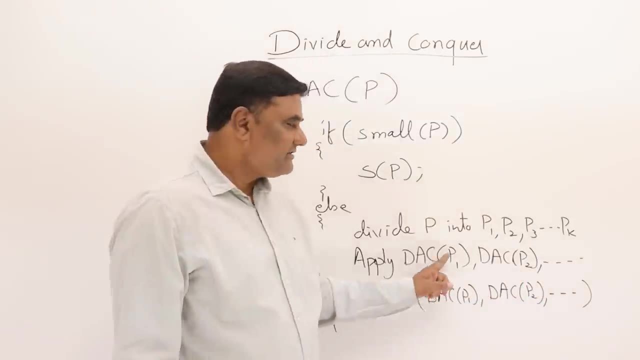 it directly. If it is large, divide the problem P into subproblems- p1, p2 to pk- and apply divide and conquer on each. This is recursive. Then, whatever the solutions you get, you combine these solutions, Okay, Combine the solutions of the results of the problem, And this is